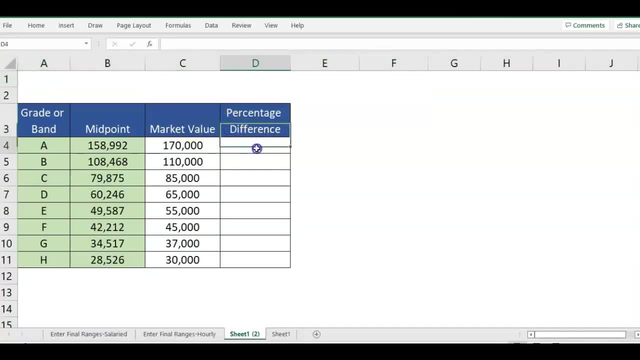 want to see what is the percentage difference. So to calculate this you first want to identify what is your old and new value. So we're gonna say the midpoint is the old value and the market value is the new value. And this is just helping with the formula so we can know We're just gonna do equal. 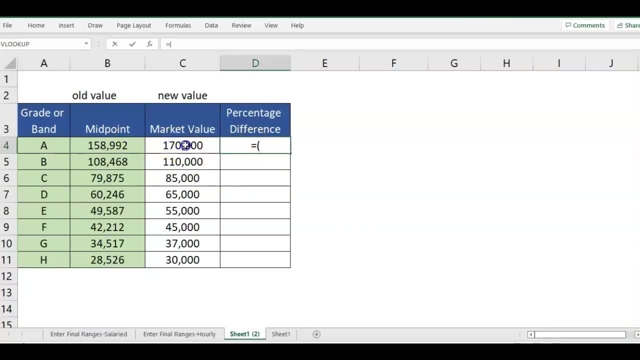 parentheses. We're gonna take the new value first, minus the old value, close parentheses, and then we're gonna divide it by the old value. So new minus old divided by old, and that is giving us the percentage difference. So you could also break that out into two cells if you wanted to just do a. 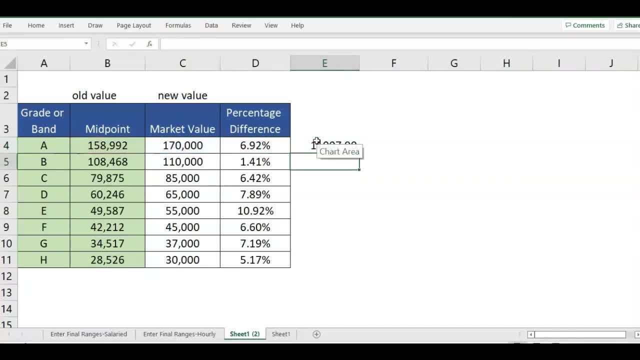 new value minus old and get a dollar amount for that, And then you can break it into two steps and you would just take that difference amount divided by original and you're gonna get the same percentage. So that's another way you could look at it, And so that's how you calculate the. 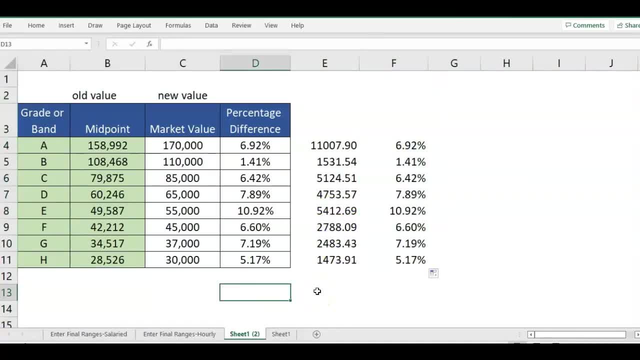 percentage difference. That was really fast. If I was looking at this for a company, I would probably look at the average, I would probably look at the average and I would look at the average. So equals average and take the average percentage difference here to see, just to see. 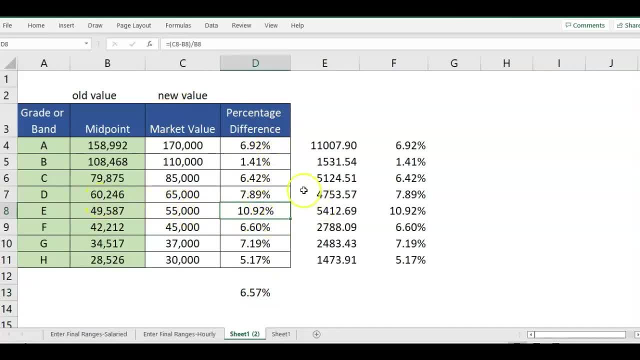 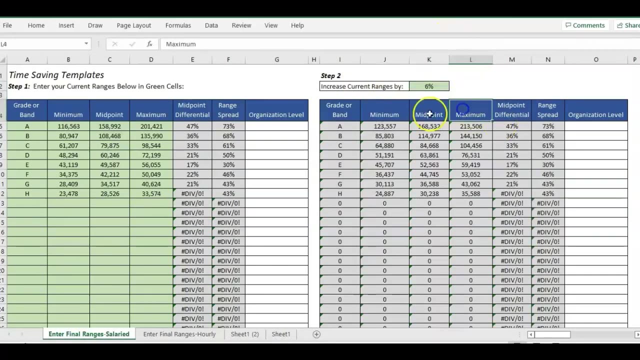 what the total average is. Some are having a larger difference than others, and then maybe that I may add this into the template. actually that may help to inform: if on average it's 6.5, maybe we would increase ranges by 6%, And so then that would update the formulas below And. 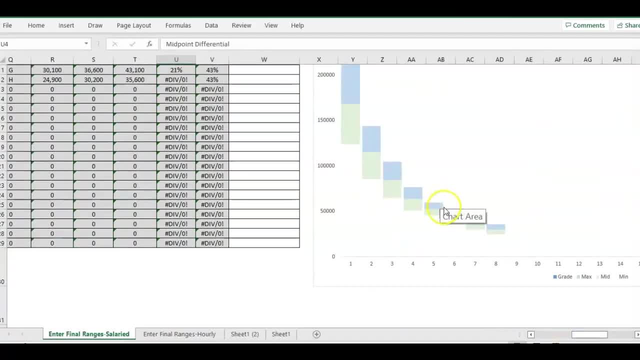 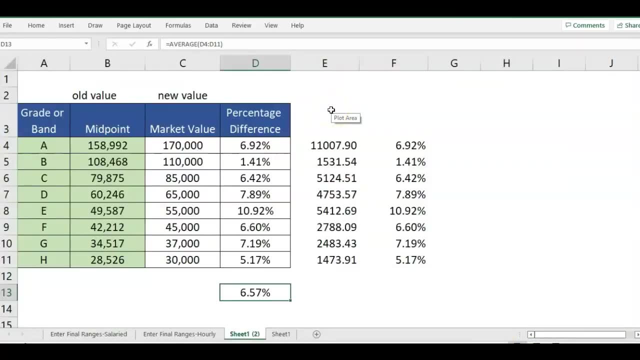 so that is part of the formula, Part of the template. the chart will update with the new ranges information. So I hope that helps next time you're looking to compare the percentage difference between two numbers. And just in case you're interested in if you work in HR or compensation, we have the salary range reset. 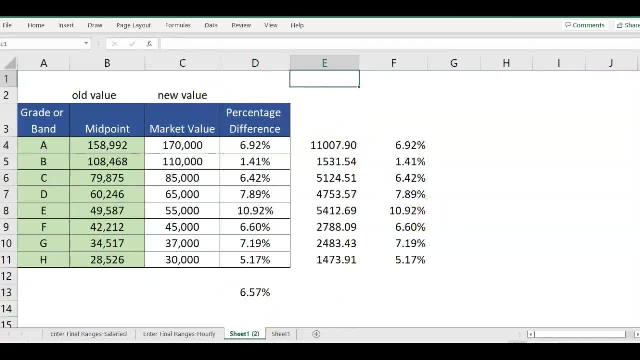 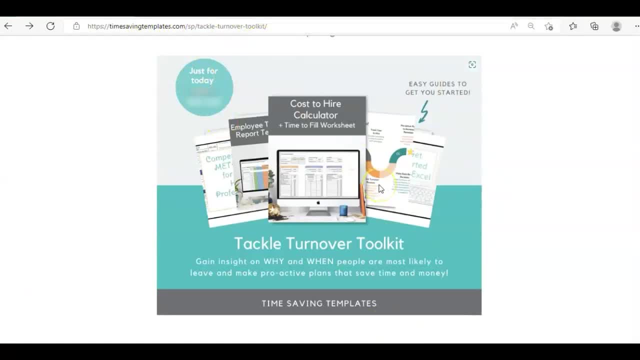 template. It's part of a turnover package actually, which you can find- I'll link to in the comments. It's part of the salary range reset template. So if you're interested in the tackle turnover toolkit, so that is going to contain several templates to track turnover cost.